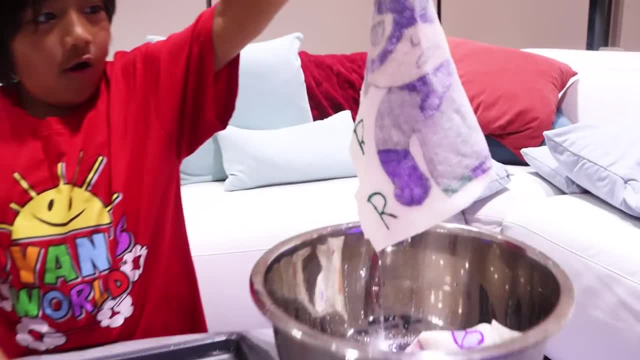 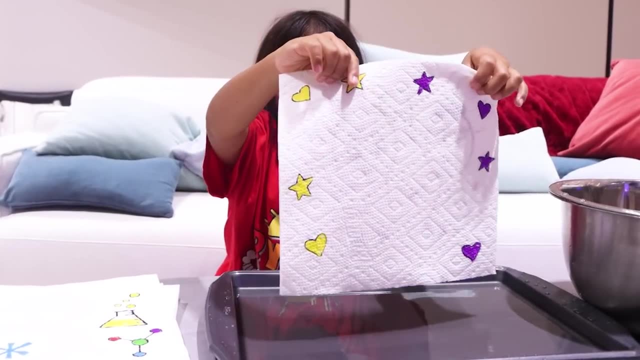 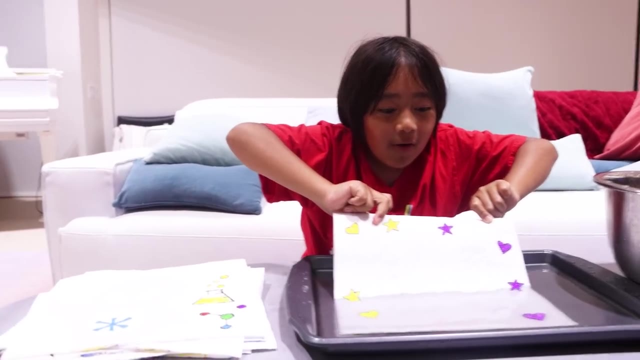 Whoa. So next is a bunch of hearts and stars. I wonder what it could be. Well, let's see. Oh, there's some feet. Oh wait, it says E and K. It's a monkey. Let me show you a better look. 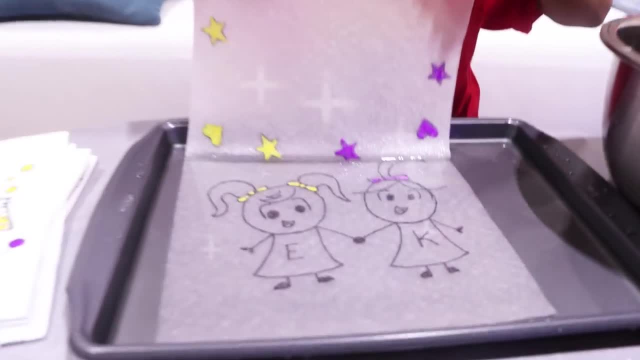 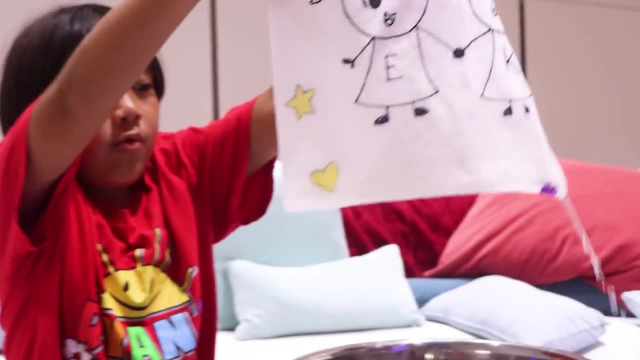 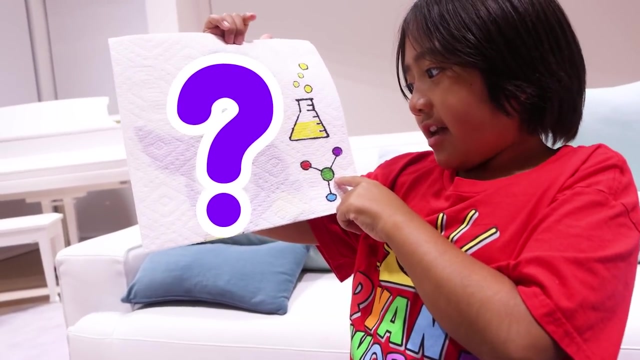 Let's see if we're right. Whoa, yeah, we were right. Okay, a monkey, you're going to go into the bowl? Hmm, I see some science stuff. Oh, and an atom and a snowflake. Hmm, I wonder who that could be. 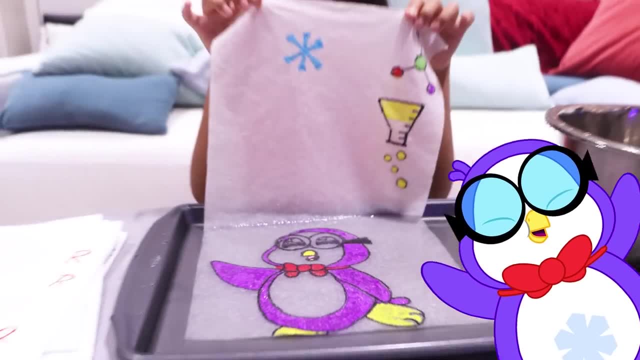 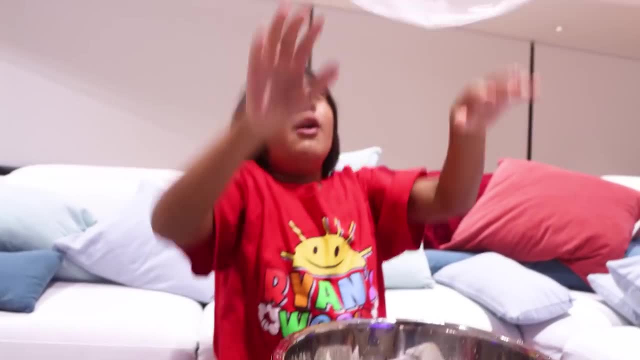 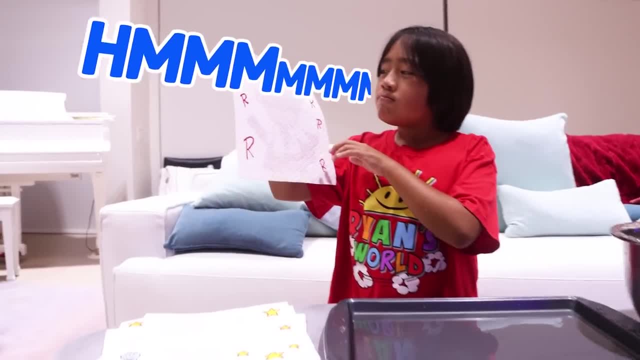 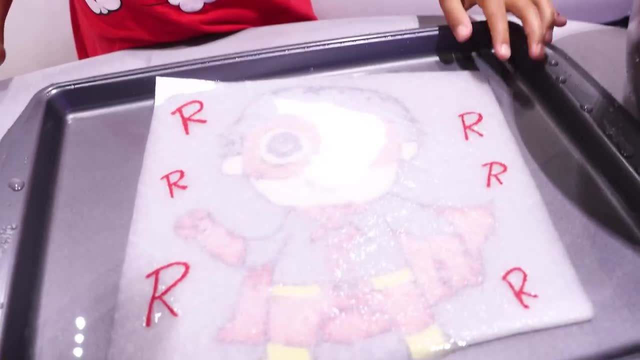 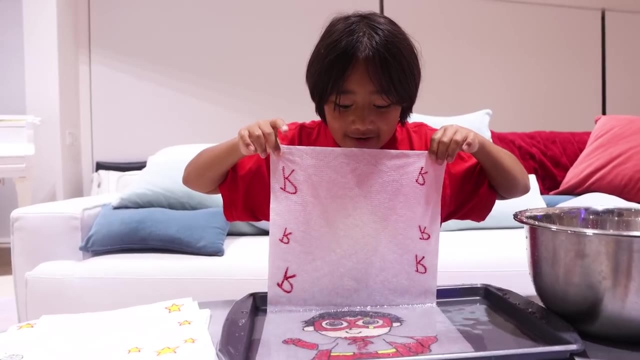 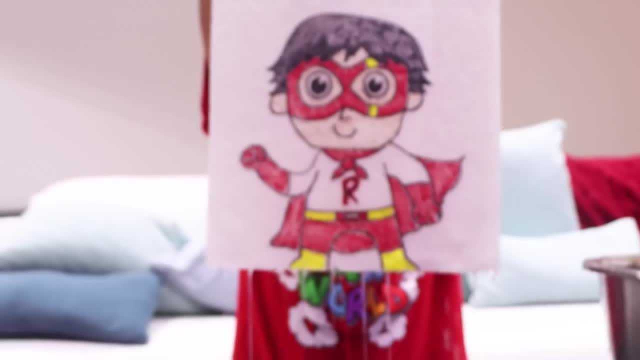 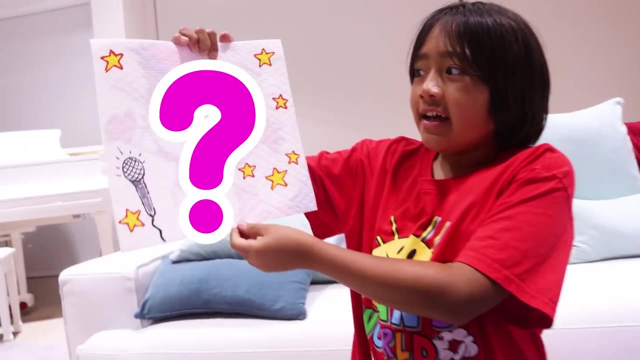 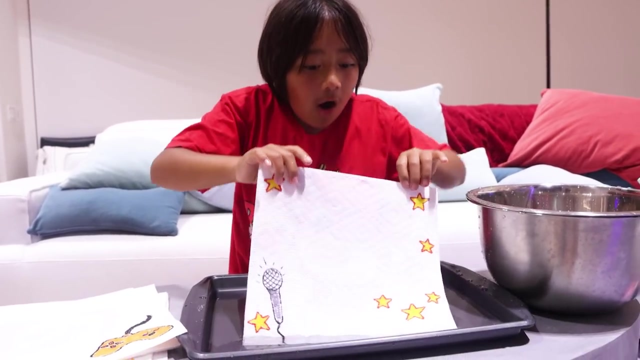 I am super, duper strong. Whoa Next, Hmm, next, who likes to sing? There's a bunch of stars too. I wonder who it could be. Let's see. Oh, who's this pink? I think it's Alphalexa. 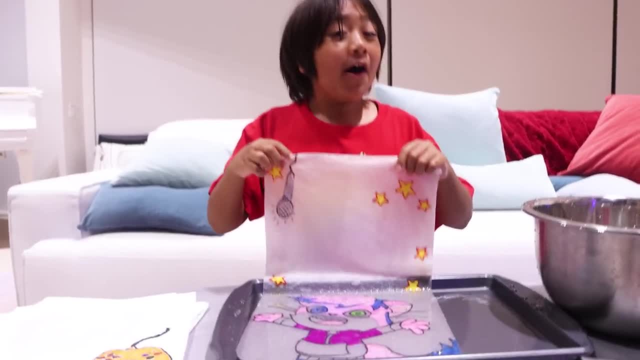 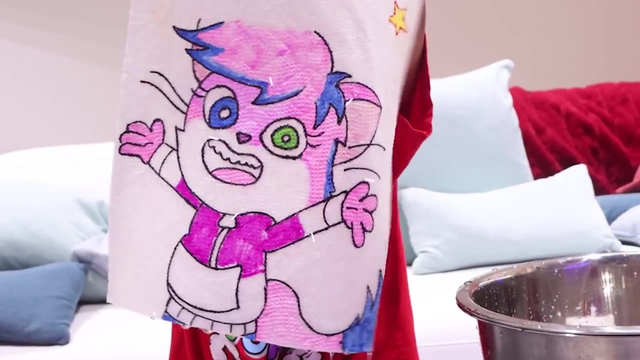 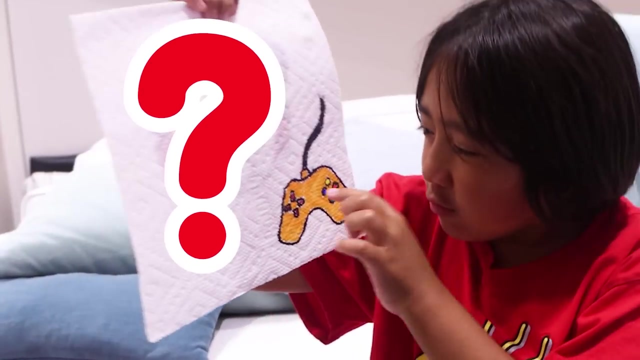 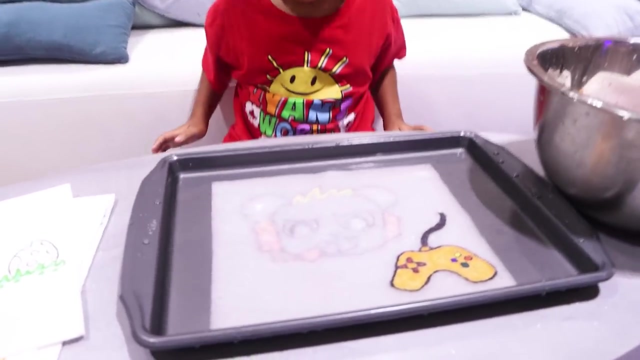 Let's see. Oh yeah, that's Alpha. Awesome. Whoa. See you guys later. Bye, Wow, A gaming controller. I wonder who that could be. Okay, Let's see. Whoa, It's Combo Panda. Whoa. 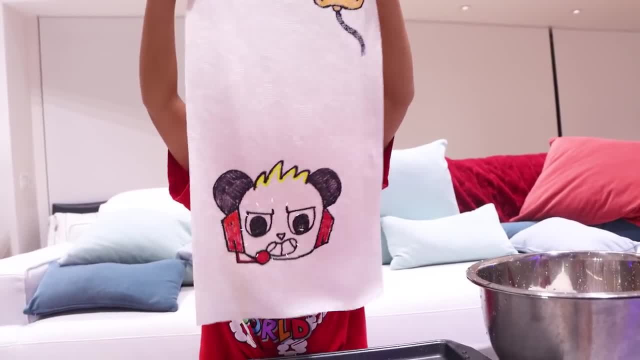 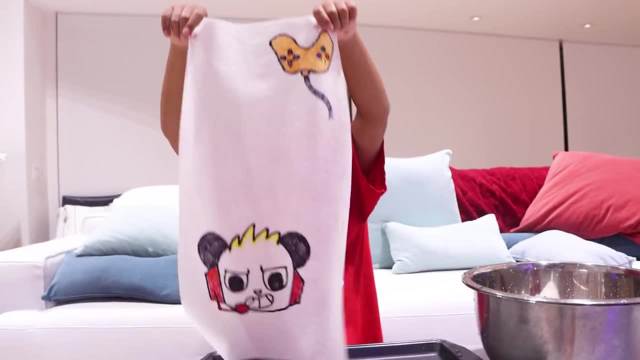 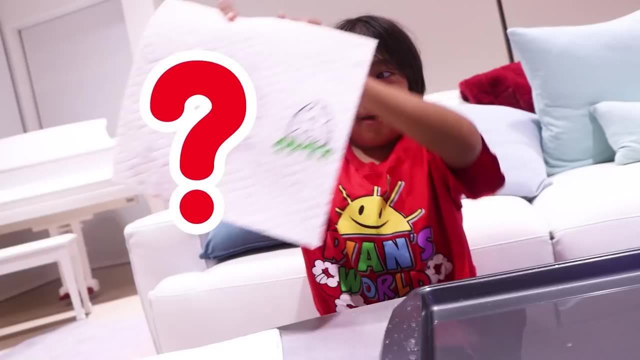 Hi guys, I am Combo Panda. Today we are going to play Roblox and we are going to do an obby And we are going to jump right here. Hmm, I wonder what's next? It's an egg. I wonder who that could be.